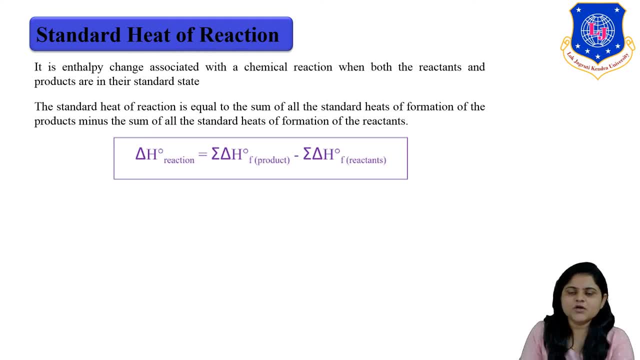 delta H of the reaction is equal to sigma delta H of the formation of the product, minus sigma delta H of the formation of the reactant. That means a standard heat of reaction is equal to summation of standard heat of formation of the reactant. 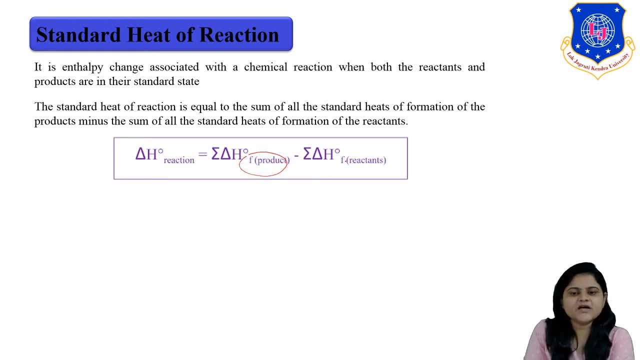 product minus summation of standard heat of formation of the reactant. Say, for example, small a into capital A plus small b into capital B gives you small c into capital C plus d into d, where small a and small b are stoichiometric coefficient of reactant A and B respectively. and 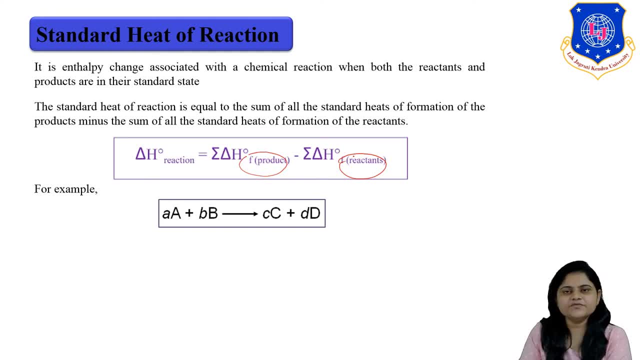 small. c and d are stoichiometric coefficient of the product c and d respectively. So in that case a delta HFA is the standard heat of formation of the component A. Similarly, this one is standard heat of formation of the component B. This one is standard heat of formation of component C. 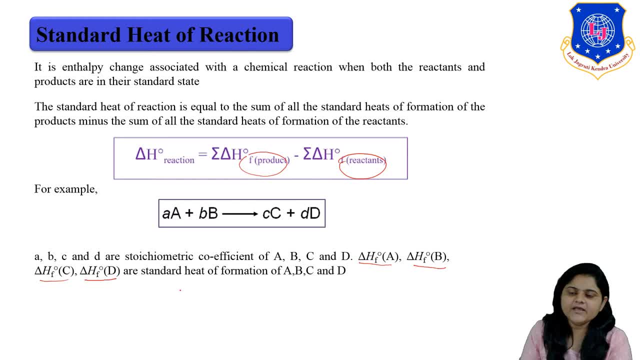 and this is standard heat of formation of component D. So in that case, standard heat of reactant A is the standard heat of formation of component B. So in that case, standard heat of reactant A is the standard heat of formation of component B. So in that case, standard heat of 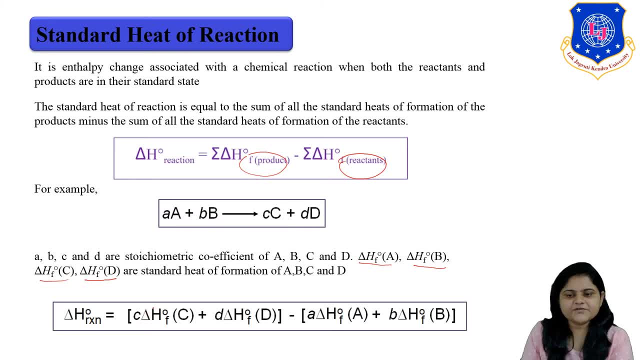 reaction is equal to a stoichiometric coefficient of the product C. That means small c into standard heat of formation of the product C plus b into standard heat. of formation of the product B minus a into standard heat. of formation of the reactant A minus b into standard heat of formation. 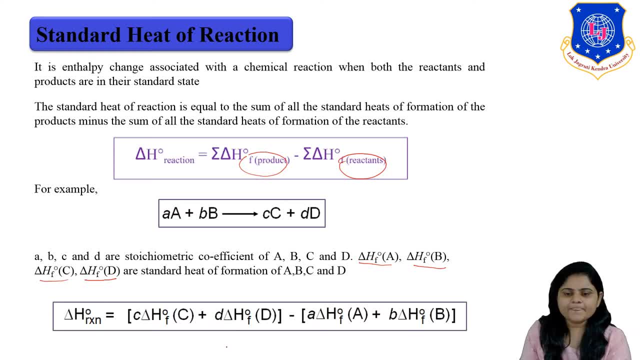 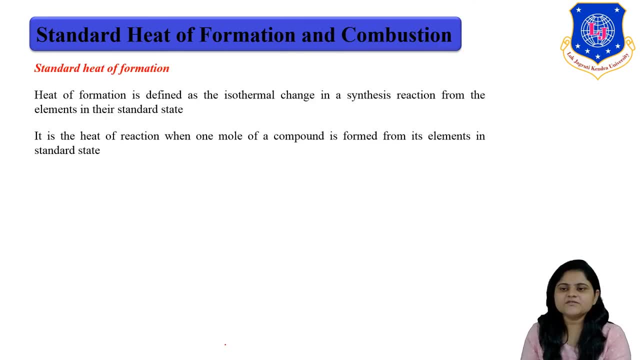 of the reactant B. So let us solve a numerical based on that and also cover a standard heat of formation and the combustion. So meaning of standard heat of formation, that means a heat of reaction when one mole of compound is formed from its element, if its elements are in. 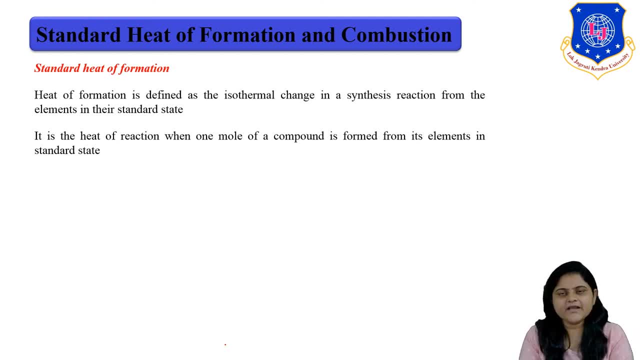 the standard state. That means if elements are in standard state and one mole of compound is formed from that element, then the heat associated with that reaction is equal to c. into standard heat of reaction is known as the standard heat of formation. That means a isothermal change when a. 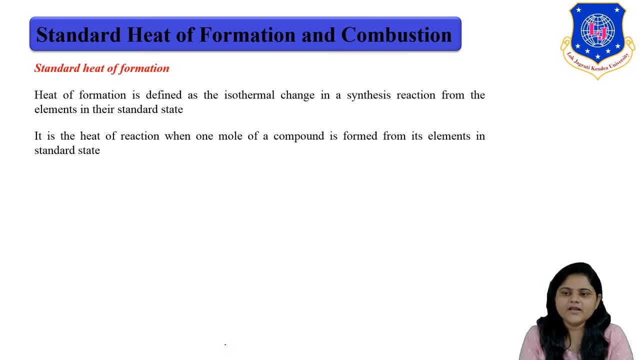 reaction is going to take place if elements are in the standard state. Now we will see the meaning of standard heat of the combustion. That means when one mole of a substance burns with the molecular oxygen to give a specific product under the standard heat of the combustion. that means 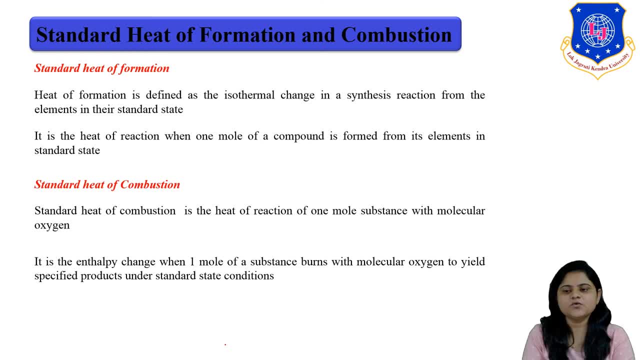 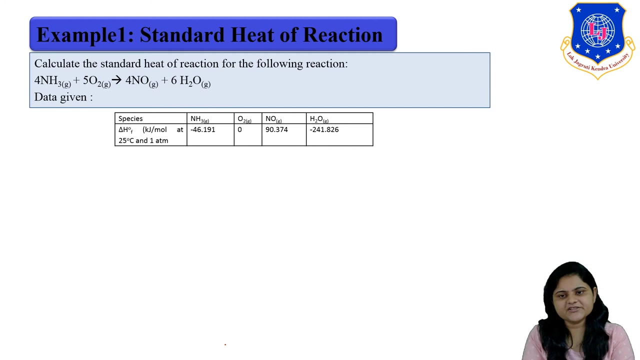 the heat associated with that is known as the standard heat of combustion. That means it is a heat of reaction when one mole of substance is going to react with a molecular oxygen and it is in its standard state. Now a numerical based on the standard heat of reaction A given data is like: 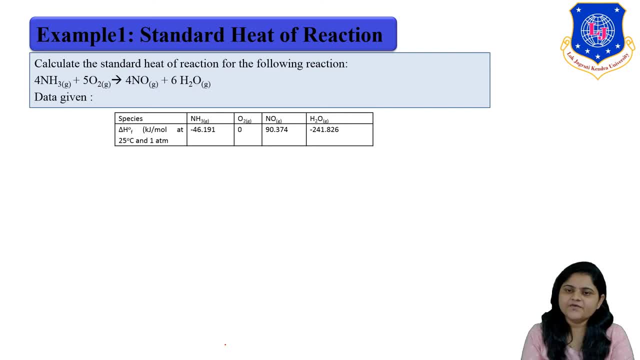 this Calculate the standard heat of combustion. So if the heat of combustion is equal to c into heat of reaction For the following reaction, NH3 plus O2 will give you NO plus H2O And for that species a standard heat of formation for NH3, oxygen NO and H2O is given to us. This standard. 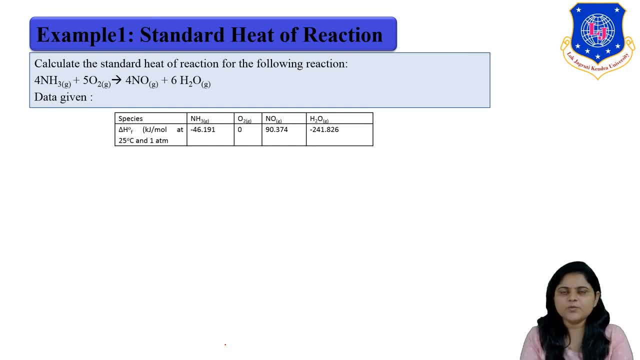 heat of formation is a condition: 25 degree Celsius and 1 atmospheric pressure. Whenever you will solve a numerical based on this standard heat of reaction, first your task is to balance this chemical reaction. So in this a chemical reaction is already balanced, So we can write. 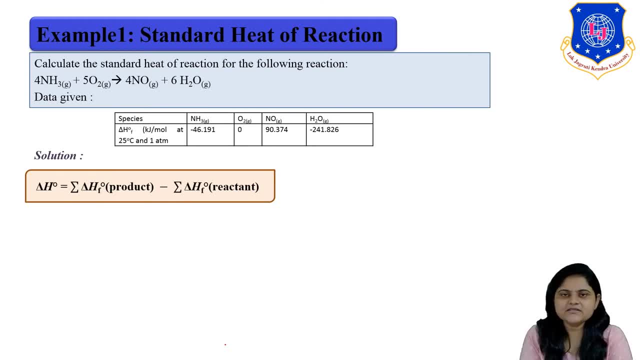 down the equation for standard heat of reaction, as this Standard heat of reaction is equal to sigma standard heat of formation of product minus summation of standard heat of formation of the reactant. So in our case, a product is this: NO and H2O, So do the summation of this along with the 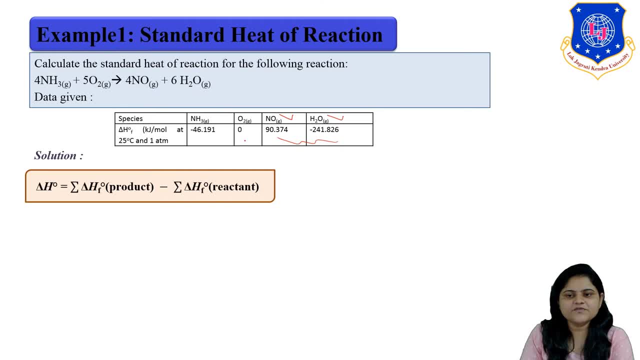 stoichiometric coefficient minus do the summation of this reactant along with the stoichiometric coefficient. So standard heat of formation is equal to this stoichiometric coefficient. 4 into standard heat of formation of NO, which is 90.374, plus 6 into standard heat of formation. 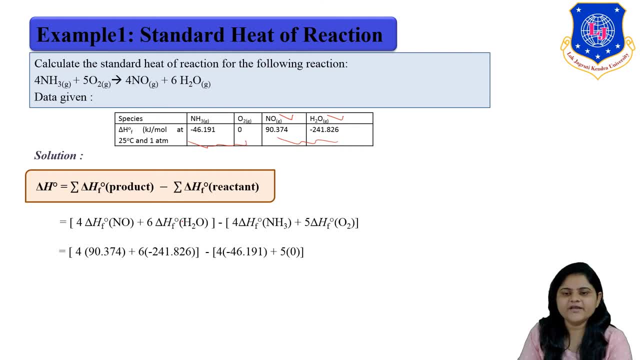 of H2O, which is minus 241.826, minus 4 into standard heat of formation of NH3, which is minus 46.191, plus 5 into standard heat of formation of oxygen, but it is 0.. To simplify this, you will get standard heat of reaction as minus 904.696 kilojoule per. 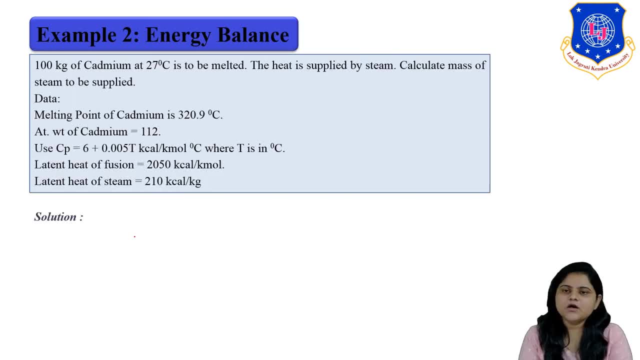 kilo mole. Now let us solve one more numerical, based on the sensible heat and latent heat of vaporization. A given data is like this: 100 kilogram of cadmium at 27. Degree Celsius is to be melted. the heat is supplied by the steam, so calculate the mass. 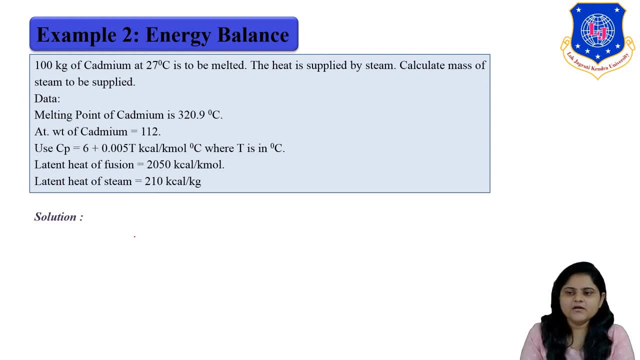 of the steam that is to be supplied. Here we need to calculate mass of steam that is to be supplied. 400 kilogram of cadmium at 27 degree Celsius that we want to melt it. A melting point of cadmium is given as 3.. 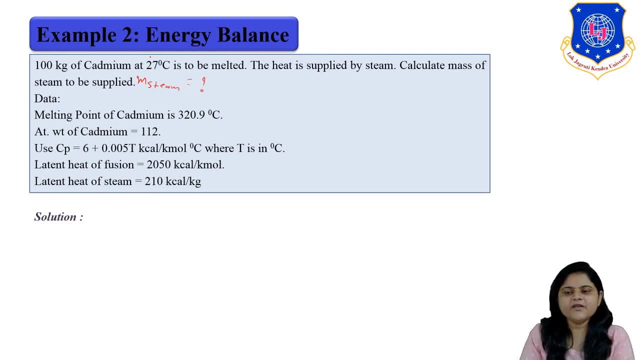 Degree Celsius is 122.9 degree Celsius. atomic weight of cadmium is given as 112. a CP equation is given like: this: CP is equal to 6 plus 0.005 T, which is in kilo calorie per kilo mole degree Celsius. 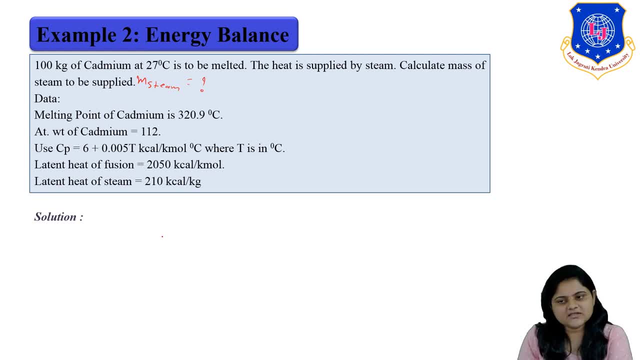 Here temperature is in degree Celsius, a latent heat of fusion is given as 2050 kilo calorie per kilo mole and latent heat of steam is given as 210 kilo calorie per kilo mole. So here we want to write 100 kilo kilomoles per kilo mole. 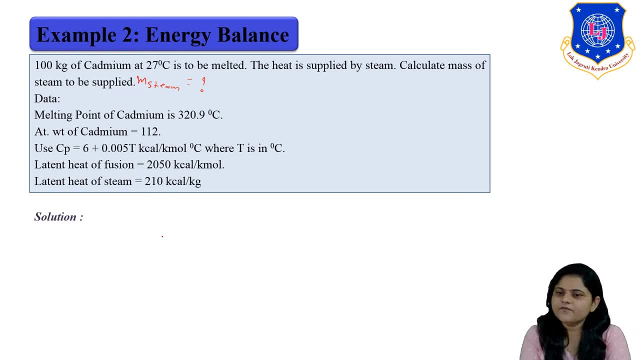 kilogram. So first we will see the meaning of the given data. Here cadmium is to be melted. present temperature of cadmium is 27 degree Celsius and melting point of melting point of cadmium is 320.9 degree Celsius. Now to do this task. 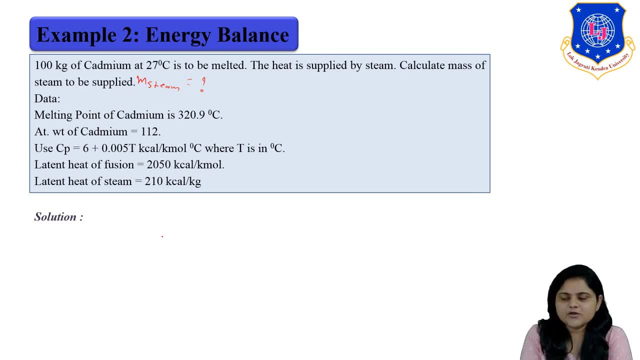 a heat is to be supplied by the steam. So we need to calculate the mass of the steam that is to be supplied in our system. So first we need to calculate amount of heat required. cube to melt the cadmium. So first to melt the cadmium here, initial temperature of cadmium is: 27 degree Celsius. So first we need to increase the temperature of cadmium from 27 degree Celsius to 320.9 degree Celsius. So for to increase the temperature of cadmium from 27 degree Celsius to 320.9 degree Celsius, some amount of heat is to be required. 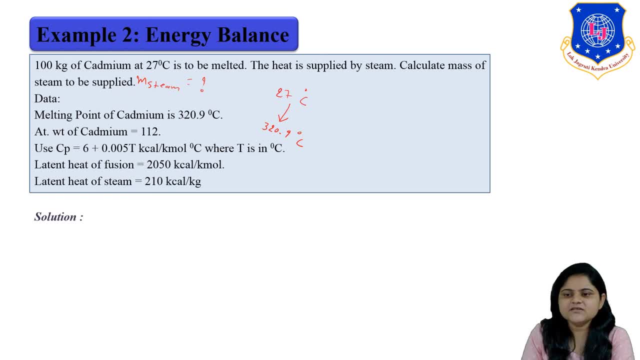 So that is to be calculated by us using this C? p equation. So, using this equation of C? p, we can calculate amount of heat required to raise this temperature. Now, along with that, a phase is going to change, So, moreover, that some amount of heat is required to change the 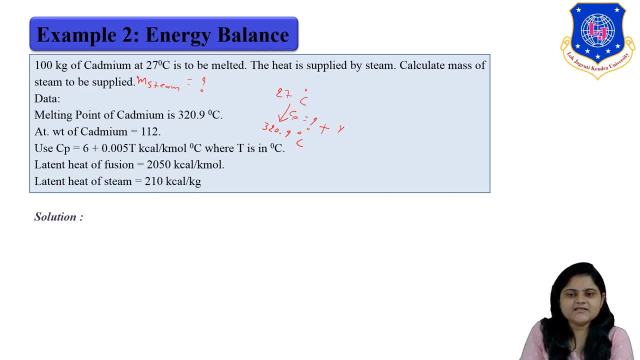 phase of the cadmium, So that heat is n into lambda latent heat of fusion of the cadmium. So first we will calculate the amount of heat required to increase the temperature. This amount of heat required to increase the temperature is known as: 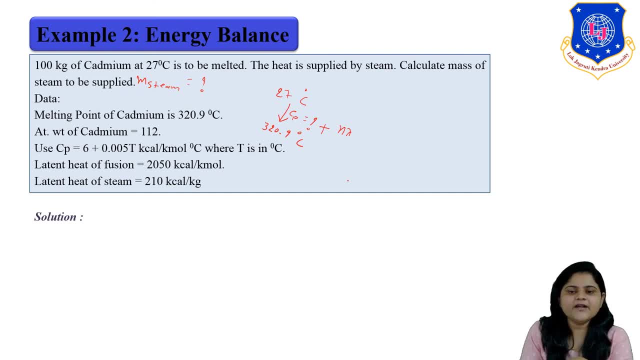 the sensible heat and amount of heat required to change the phase of the substance is known as the latent heat of vaporization. So the total heat required is the summation of heat required to change the temperature. that means a sensible heat plus latent heat of vaporization to change. 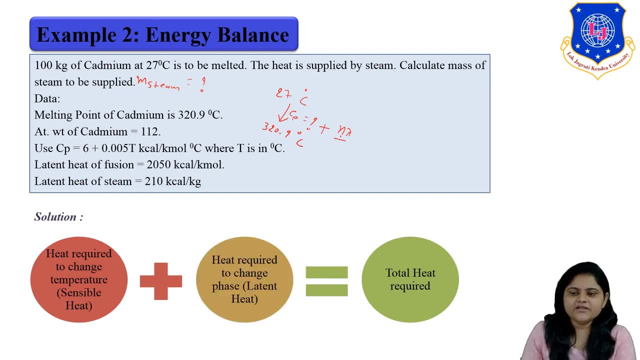 the phase of the cadmium. So in this case, first we need to calculate this sensible heat and we need to calculate the amount of latent heat. Sensible heat can be calculated by using this equation: integration of T 1 to T 2, C, p into D T, and latent heat that can be calculated by using the 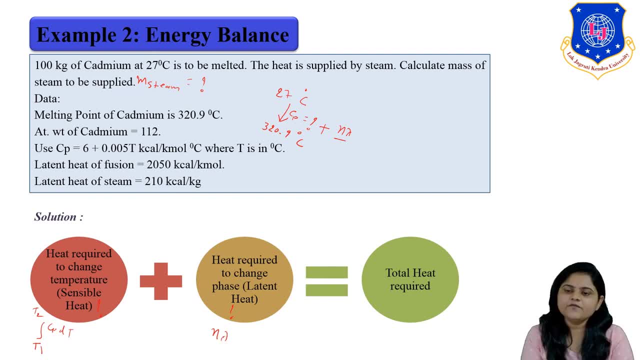 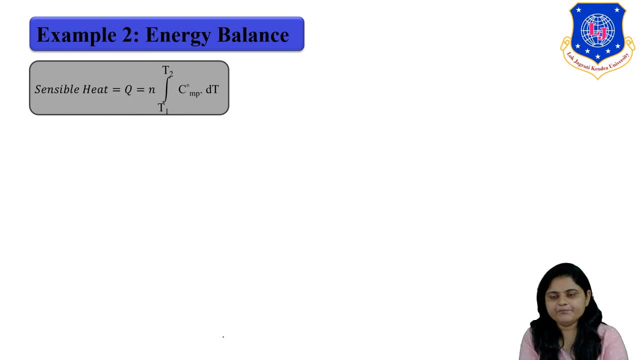 and lambda. Here lambda is the latent heat of fusion. So let us calculate sensible heat required of cadmium. This is the given equation. n is equal to number of moles. Here mass of cadmium is given as 100 kilogram divided with the molecular weight, you will get moles of cadmium as 0.892 kilomole. 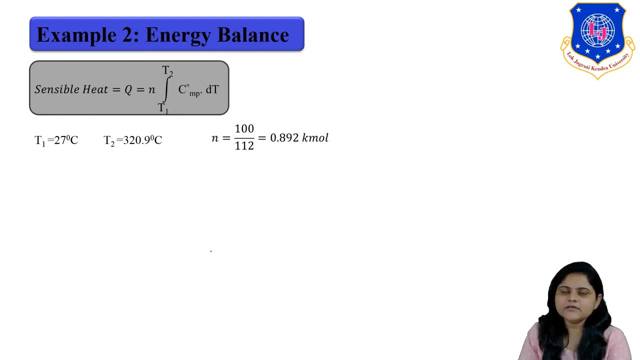 Integrate this equation with temperature T 1 and T 2.. The equation of C p is given like this: 6 plus 0.005 T. Now integrate this equation. you will get 0.892 into bracket 6, into T 2 minus T 1 plus 0.005, to T 2 square minus T 1 square. Put the 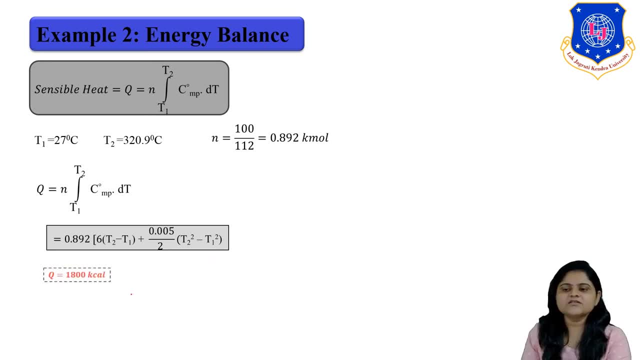 value of T 1 and T 2. in this equation you will get the answer of Q as 1800 kilocalorie. Here Q is amount of heat required to increase the temperature of cadmium from 27 degree Celsius to 320.9 degree Celsius. 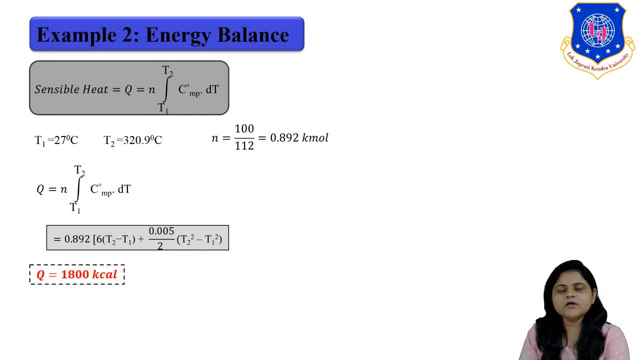 Still, some amount of heat is required to change the phase of the cadmium. So heat required to change the phase- that means latent heat- is equal to n into lambda. Here lambda is the latent heat of fusion of the cadmium. n is equal to 0.892, lambda is 2050.. So you will get 1828.6 kilocalorie. 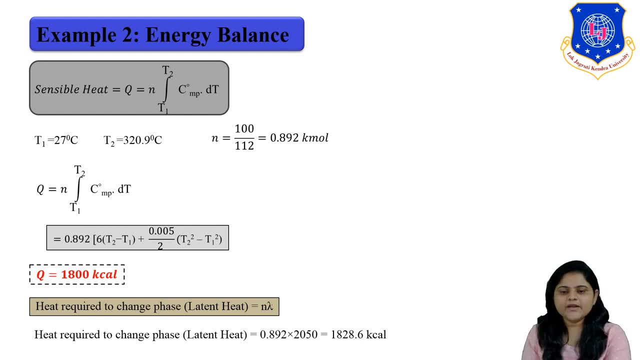 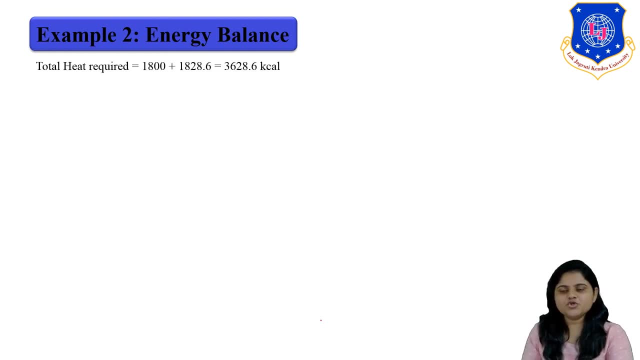 So this 1800 kilocalorie plus 1828.6 kilocalorie is the latent heat of fusion of the cadmium. So total heat required by the cadmium, So total heat required by the cadmium is 3628.6 kilocalorie. 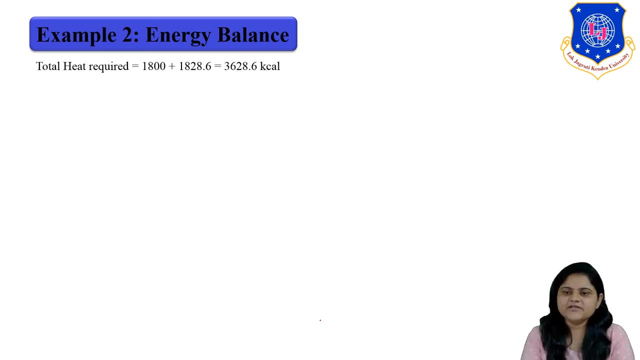 Now this heat requirement, 3628.6 kilocalorie, is to be fulfilled by a supply of the steam. So a steam is supplied to change the temperature as well as the phase change. So this, let us take that heat supplied by the steam is m into lambda. So here, 3628.6 is the total heat required. 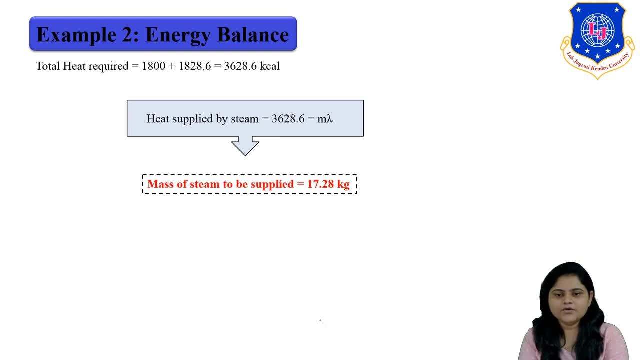 Lambda is the latent heat of vaporization of the water. So the mass of steam to be supplied is 17.28 kilogram. So this was all about today's session of material and energy.